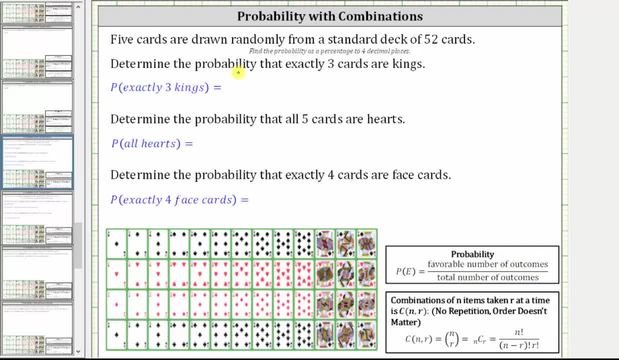 divided by the total number of outcomes. Let's begin by determining the total number of possible outcomes when drawing five cards from a deck of 52 cards, Because the order does not matter. the number of ways of selecting five cards from 52 cards is 52. choose five. 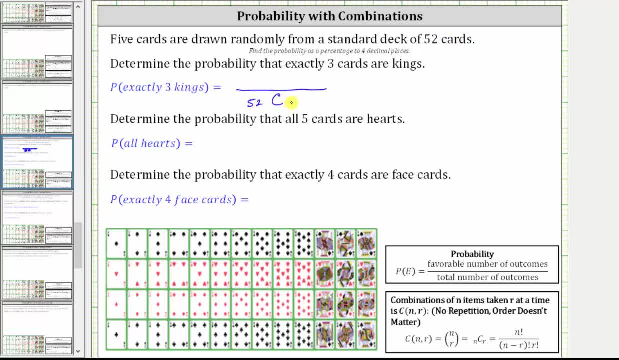 Again, we use a combination because the order does not matter, And now the favorable number of outcomes is going to be the number of ways we can select three kings from the kings in the deck, and then times the number of ways we can select two cards that are not kings from the deck. 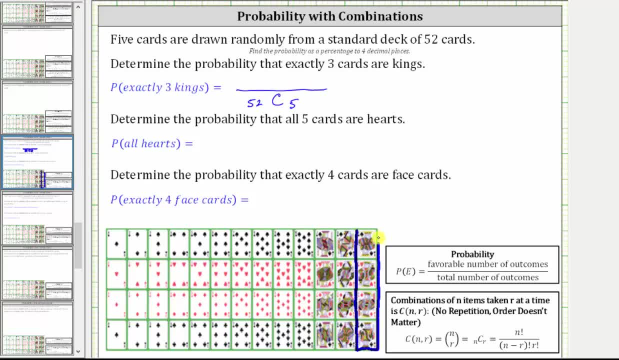 And there are four kings in the deck and therefore the number of ways of selecting three kings from four kings is: four choose three, And then we have times the number of ways we can select two cards from the deck that are not kings. Well, if there are four kings in the deck, 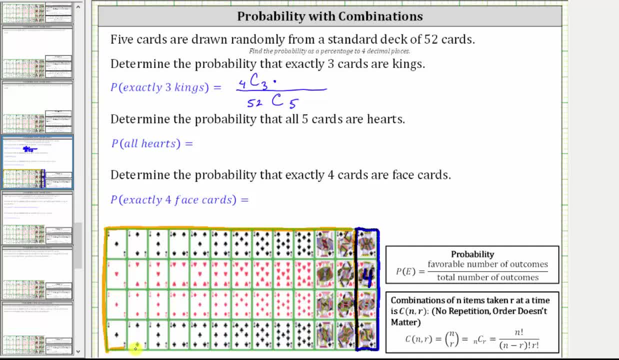 then there must be 52 minus four or 48 cards that are not kings, And therefore the number of ways of selecting two cards that are not kings is: 48 choose two. So the number of favorable outcomes is equal to four. choose three times 48, choose two. 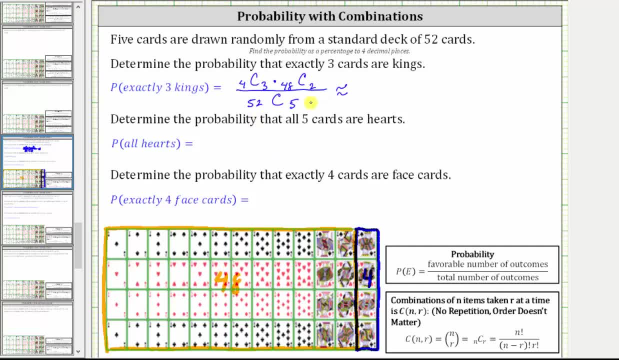 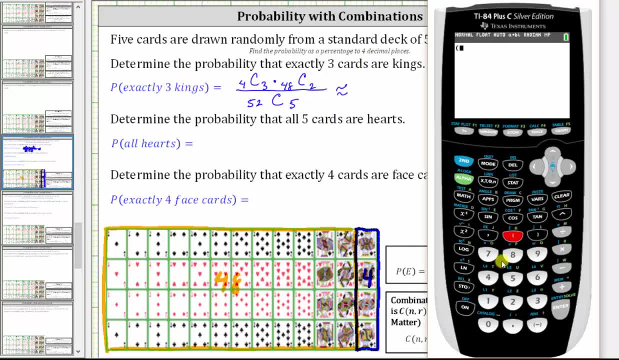 And now let's evaluate this on the calculator. And again we'll have to get the decimal to six decimal places, so the percentage is accurate to four decimal places. We need the numerator in parentheses, so we have open parenthesis. four choose three. 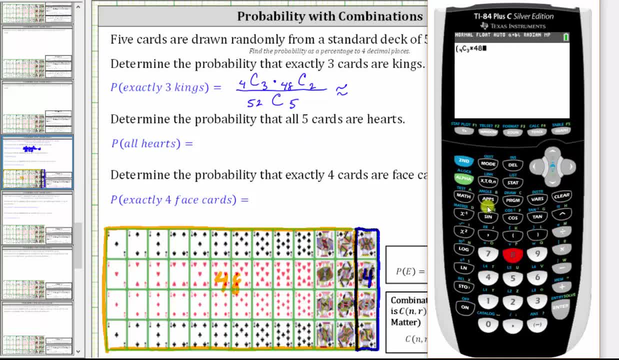 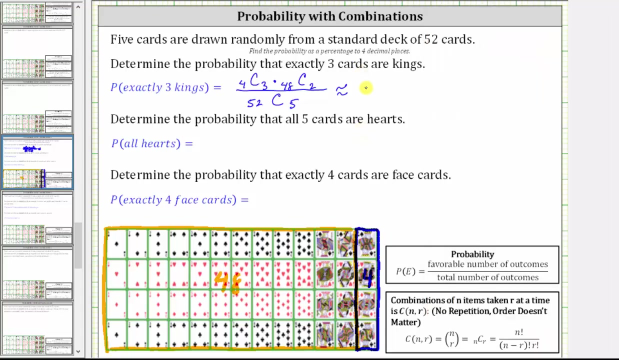 right arrow times. 48. choose two right arrow close parenthesis and this is divided by: in parenthesis 52. choose five, Which, to six decimal places, is approximately 0.001736.. Which is the percentage is 0.1736%. 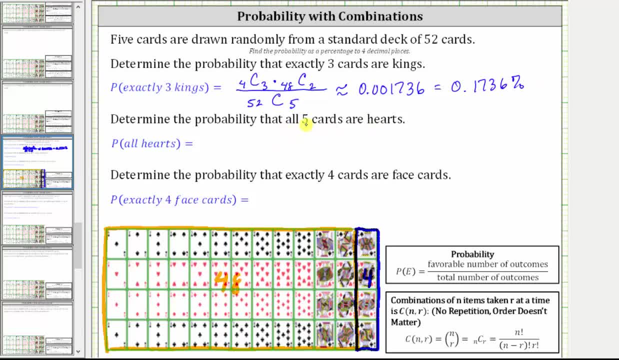 Next we're asked to find the probability that all five cards are hearts And again the total number of outcomes is going to be 52. choose five. The favorable number of outcomes is equal to the number of ways we can select five hearts from the hearts in the deck. 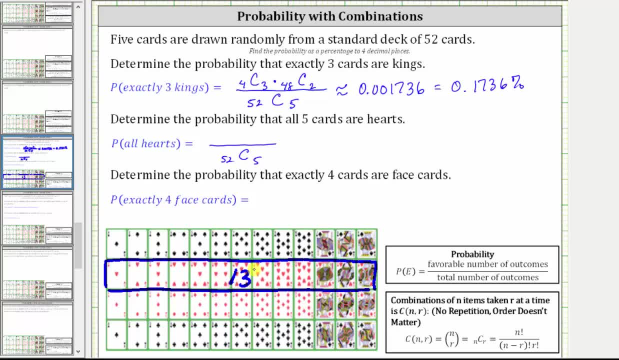 And since there are 13 hearts in the deck, the number of ways of selecting five hearts from 13 hearts is 13: choose five. And this does accommodate for all five cards being drawn And therefore this quotient is the probability. So, going back to the calculator, 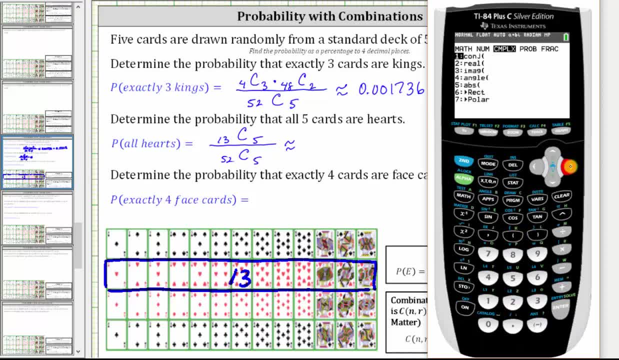 we have 13. choose five. divided by 52, choose five. Notice how this is giving us scientific notation. This means 4.9.. 4.95, et cetera, times 10, raised to the power of negative four. 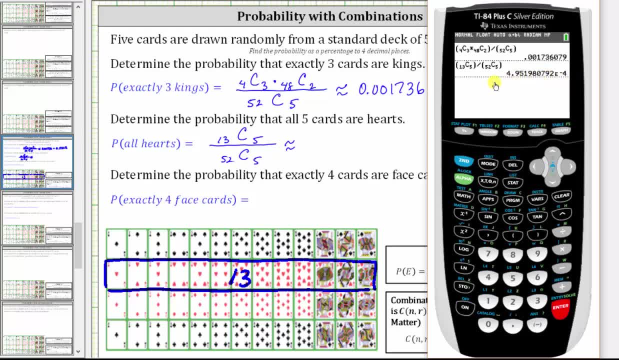 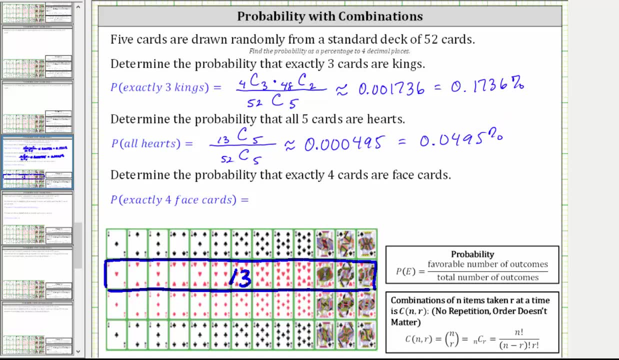 To convert to a decimal, we would move the decimal point four places to the left, which would give us 0.000495, to six decimal places, Which is equal to 0.0495%. Again, the calculator gave us approximately 4.95. 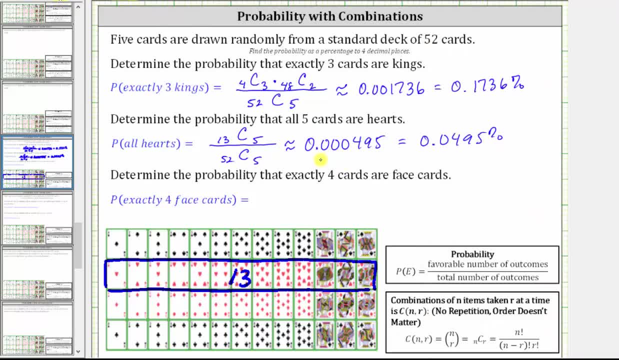 times 10 to the negative four, Which is equal to 0.000495.. Notice how to go from scientific notation to decimal notation. we move the decimal point four places to the left because the exponent was negative four For the last example. 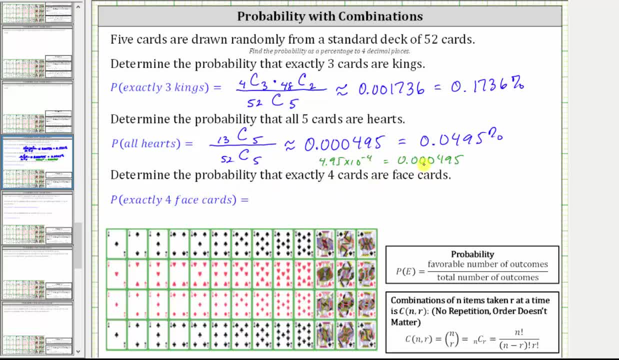 we're asked to find the probability that exactly four cards are face cards, which means four cards will be face cards and one card will not be a face card. The whole number of possible outcomes is still going to be 52. choose five, And now for the favorable outcomes. 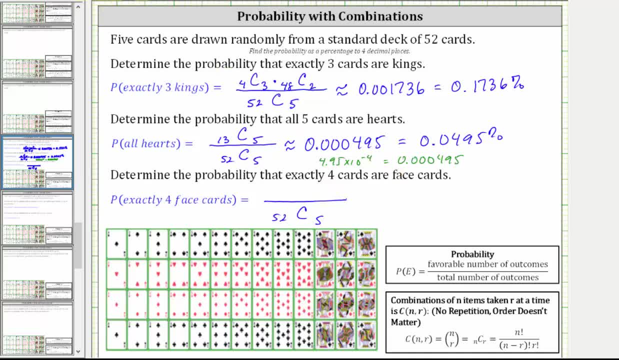 let's first determine how many ways we can select four face cards from the 12 face cards in the deck. Because there are 12 face cards in the deck, the number of ways of selecting four face cards is 12. choose four, Then we have to multiply this by the number of ways of. 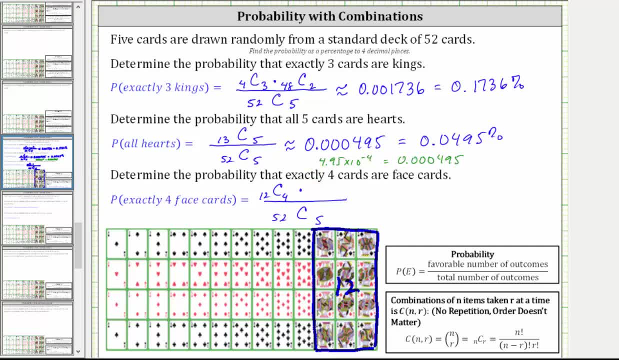 selecting one card that is not a face card, And the number of cards that are not face cards is equal to 52 minus 12 or 40. And therefore, the number of ways of selecting one card that is not a face card is 40. choose one.